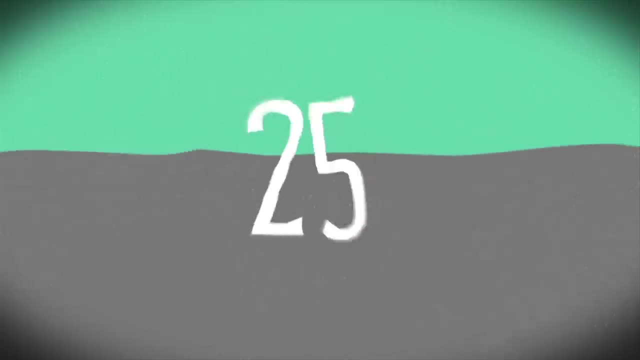 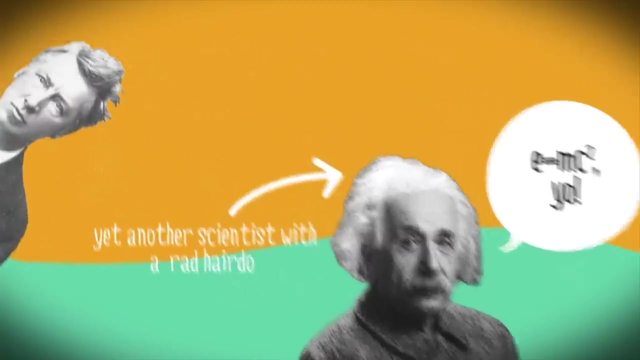 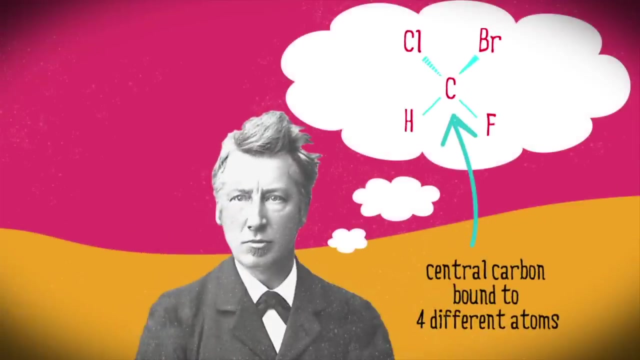 of a tetrahedron. It would take over 25 years for the quantum revolution to theoretically validate his hypothesis, but Van't Hoff supported his theory. using optical rotation, Van't Hoff noticed that only compounds containing a central carbon bound to four different atoms. 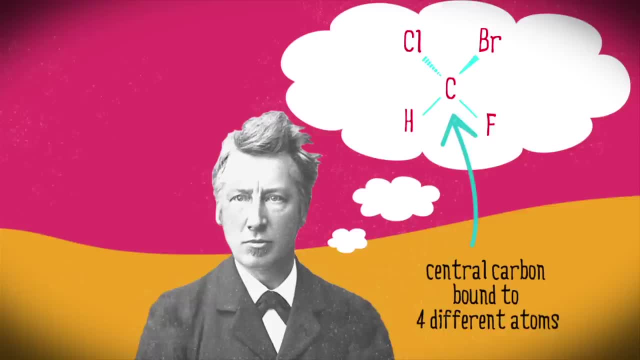 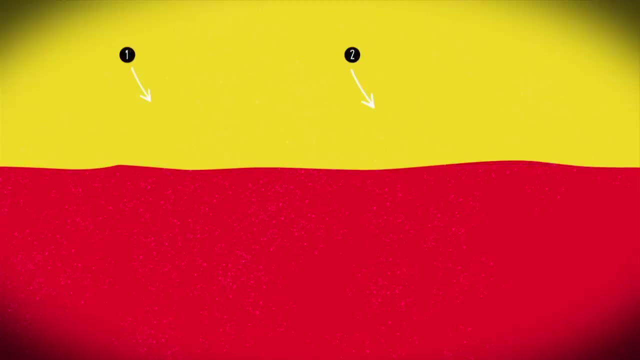 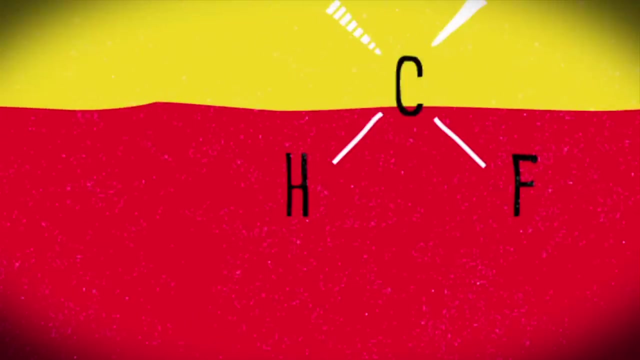 or groups, rotated plane, polarized light. Clearly there's something unique about this class of compounds. Take a look at the two molecules you see here. Each one is characterized by a central tetrahedral carbon atom bound to four different atoms. We might be tempted to conclude that the two molecules are the same if we just concern. 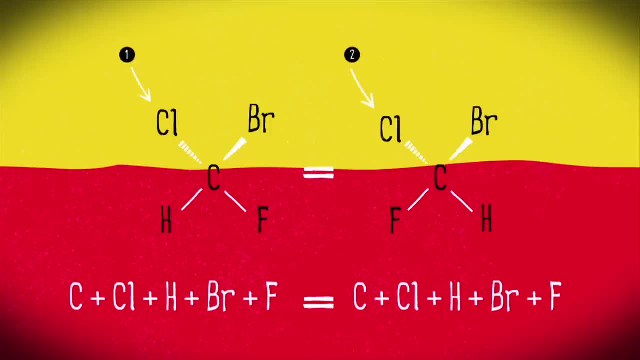 ourselves with what they're made of. However, let's see if we can overlay the two molecules perfectly to really prove that they're the same. We have free license to rotate and translate both of the molecules into the same form. We have a free license to rotate and translate. 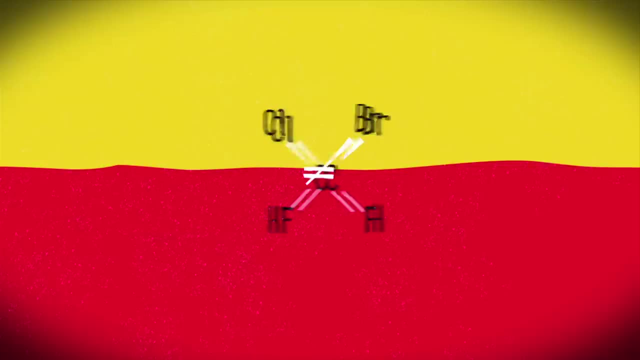 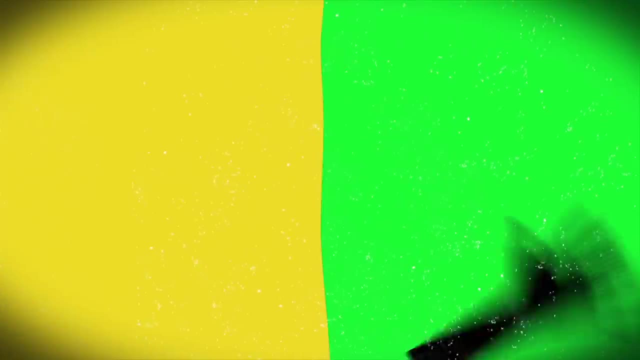 both of the molecules into the same way, we can remove those below each of the bounds as we wish. Remarkably, though, no matter how we move the molecules, we find that perfect superposition is impossible to achieve. Now take a look at your hands. Notice that your two hands have all the same parts: a. 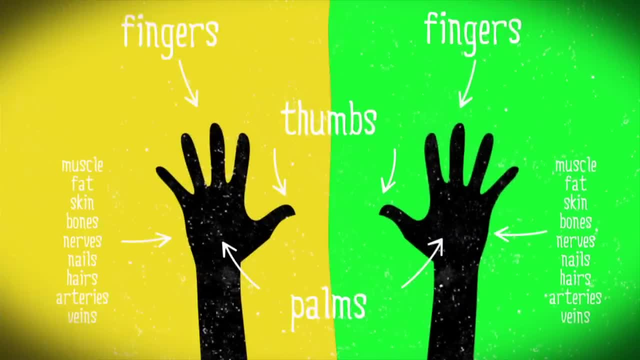 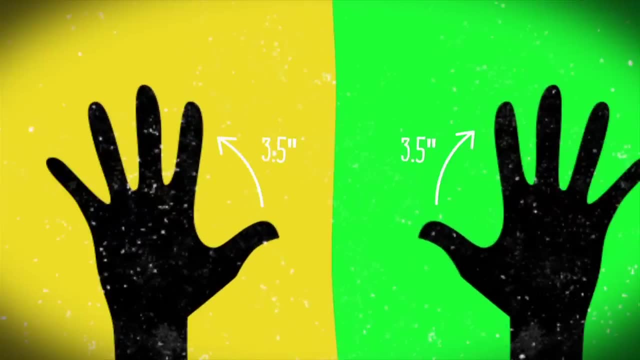 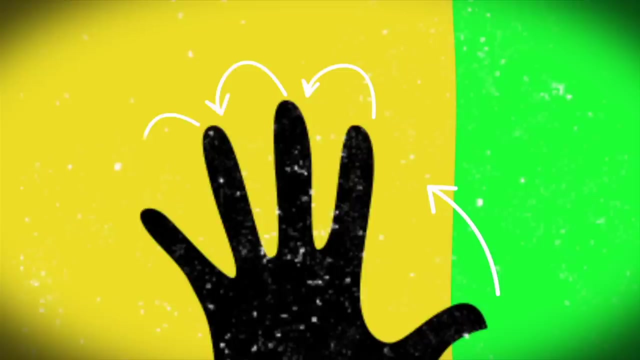 thumb fingers, a palm, etc. Like our two molecules under study, both of your hands are made of the same stuff. Furthermore, the distances between stuff in both of your hands are the same: The index finger is next to the middle finger, which is next to the ring finger, etc. 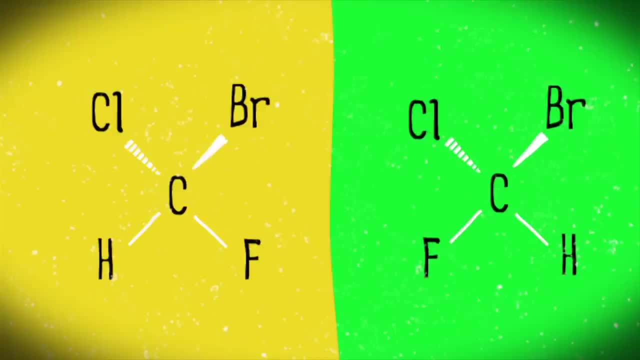 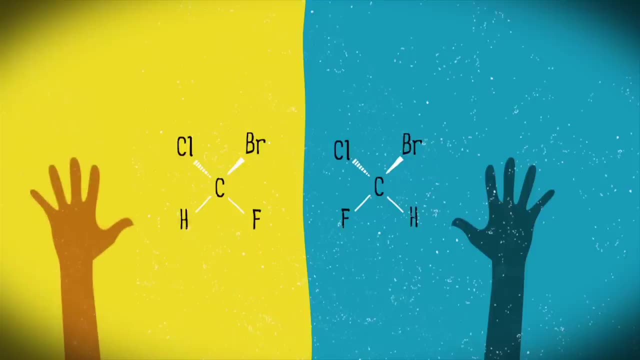 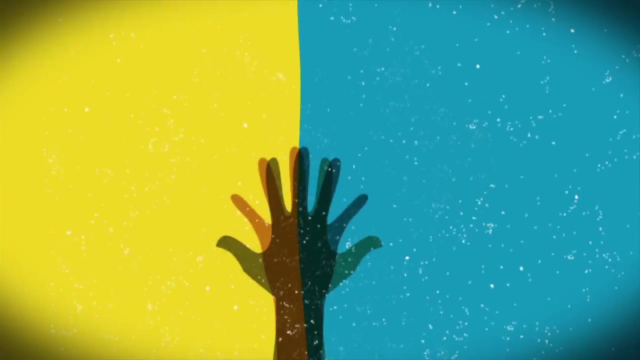 The same is true of our hypothetical molecules. All of their internal distances are the same, Despite the similarities between them. your hands and our molecules are certainly not the same. Try superimposing your hands on one another, Just like our molecules from before. you'll find that it can't be done perfectly. 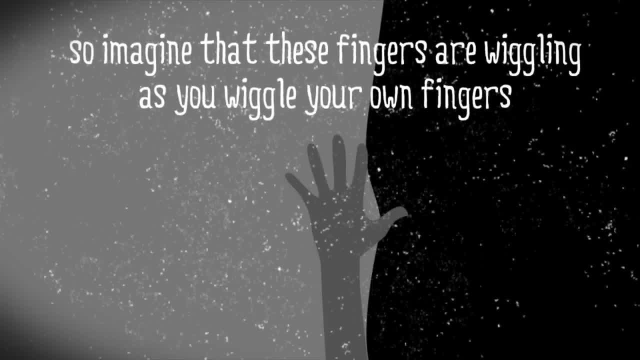 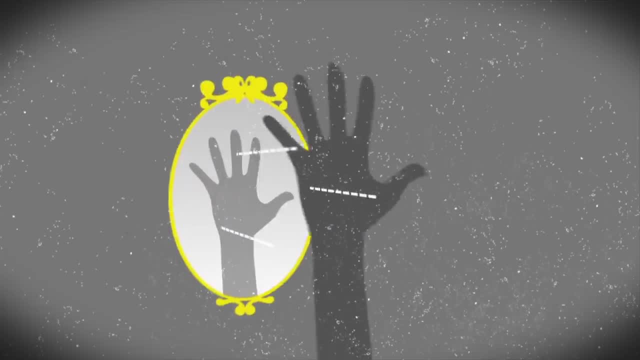 Now point your palms toward one another. Wiggle both of your index fingers. Notice that your left hand looks as if it's looking in a mirror at your right. In other words, your hands are mirror images. The same can be said of our molecules. 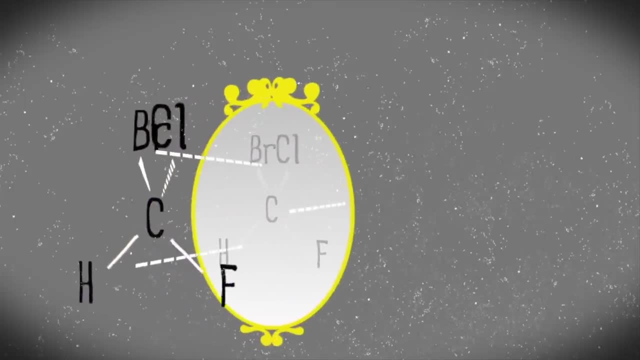 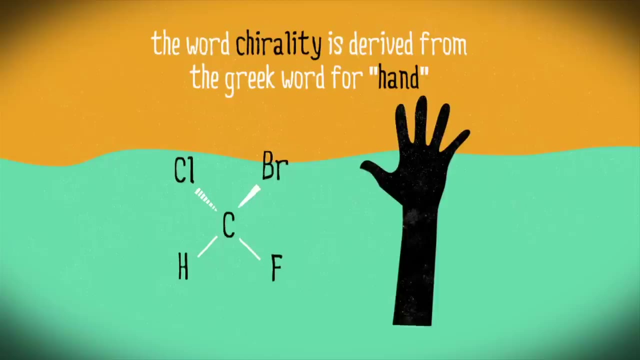 We can turn them so that one looks at the other as in a mirror. Your hands and our molecules possess a spatial property in common called chirality or handedness. Chirality means exactly what we've just described: A chiral object. It's not the same as its mirror image.